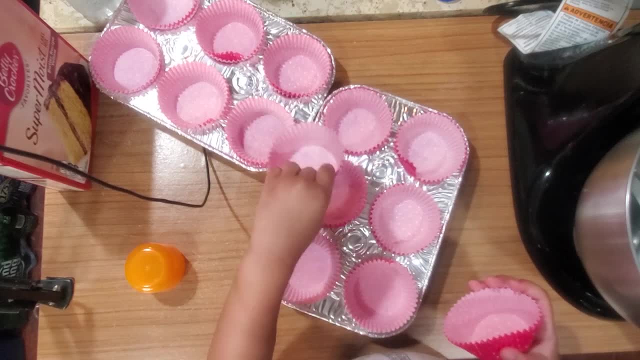 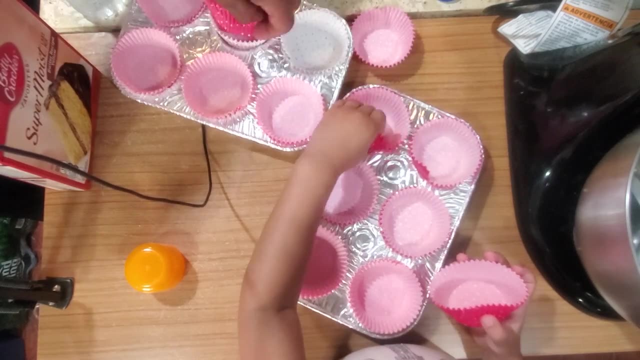 But we're spraying a little bit of this in each of the cupcakes so that the when we go to take the cupcakes out, right, they don't stick together. What are we going to do? They'll be easy to take out, Daddy. 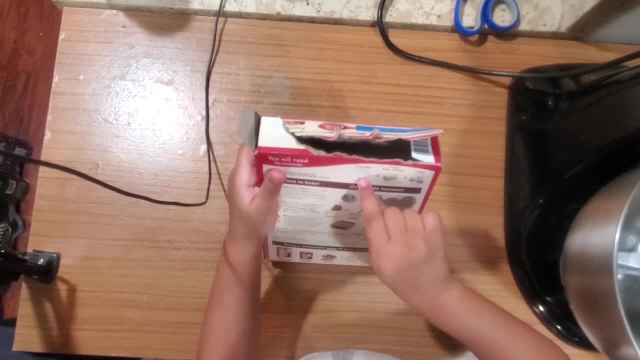 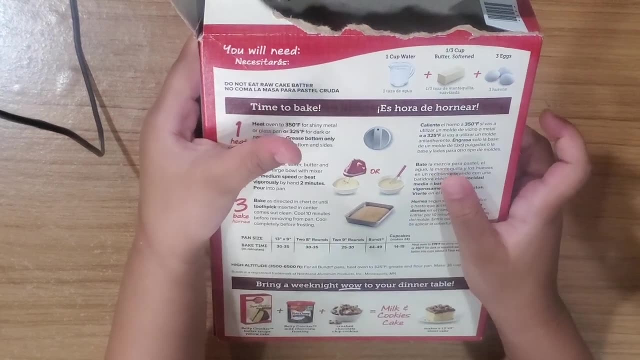 I apologize. Daddy, can you get me a cup of water? We do, I got all of that And a cup of butter, Mm-hmm. A cup of eggs. Look, We got some eggs. Look, we got the eggs warming up over here. 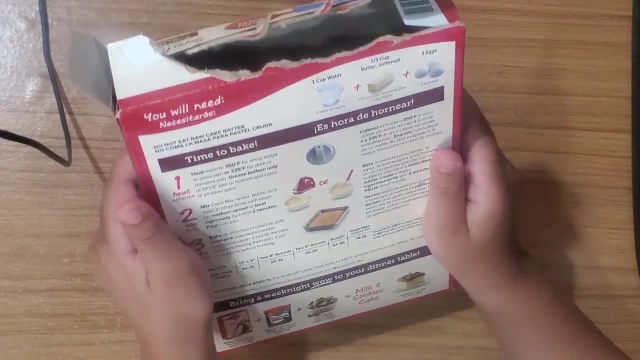 I'm going to bring it so you can show the video, So you can tell them The recipe has what again, What do you need in the recipe? Eggs, Okay. So look, let's put the eggs there. You see, the eggs. 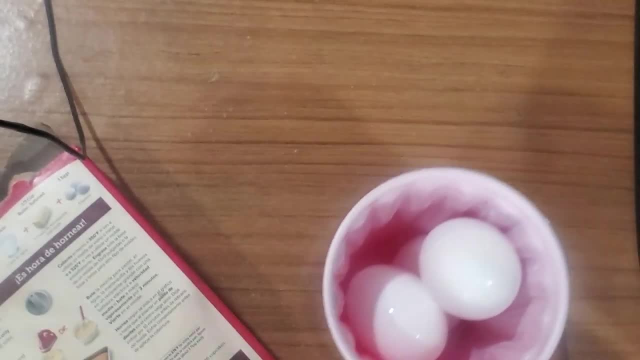 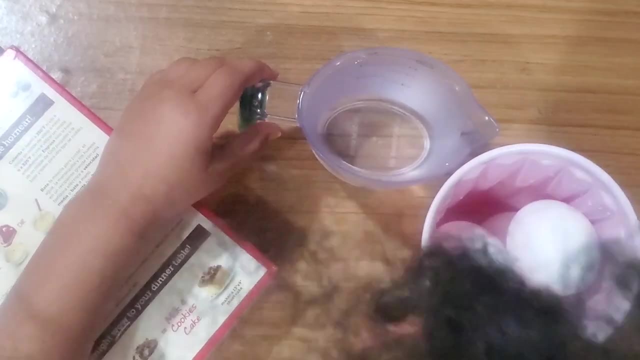 Very good. And then the recipe also has what else? Um, A cup of water, A cup of agua. There you go, your cup of agua. Now we're going to pour it- Not yet We're going to pour everything in there- but you got to give it and we got to wait a minute because we're not done yet. 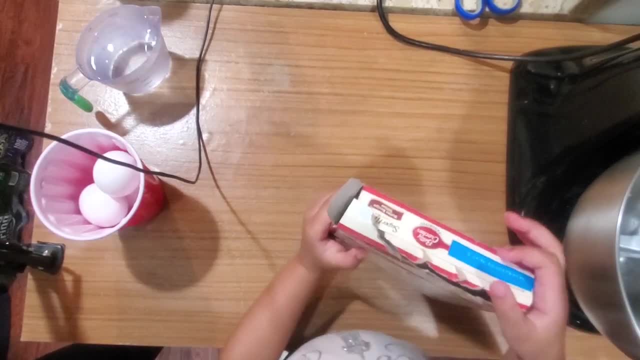 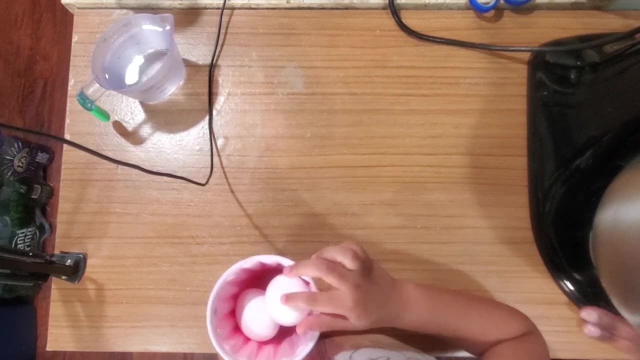 And a cup of butter. Here we go. We need a cup of butter now. I'm going to bring you the butter, Don't worry, but let's get the blender over here. Let's move the blender, Excuse me. Let's move the blender. 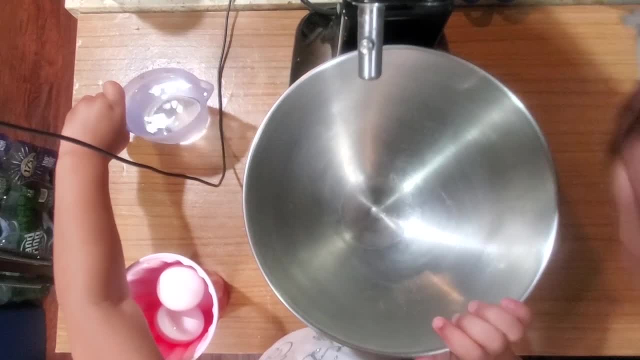 And now let's put some more butter. Let's move this out of the way. Let Daddy take that off. No, no, no, No, agua first. No, we don't do agua first, First, we're going to put this right. 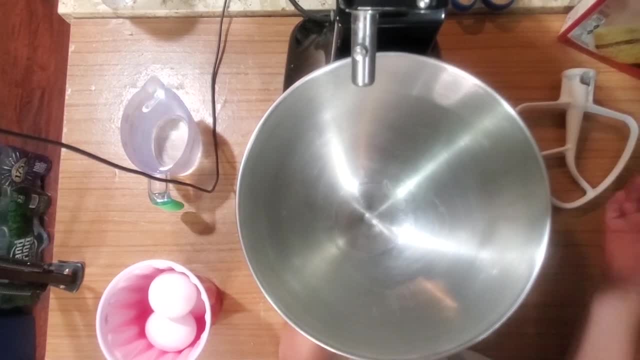 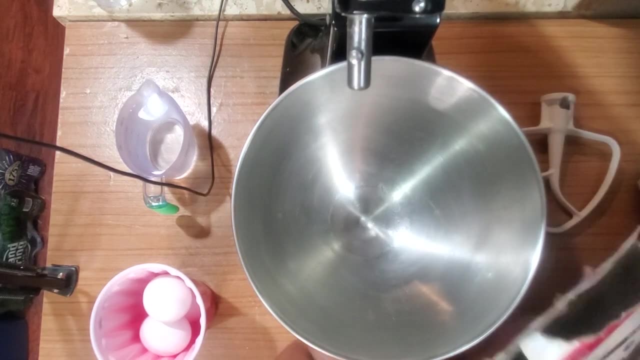 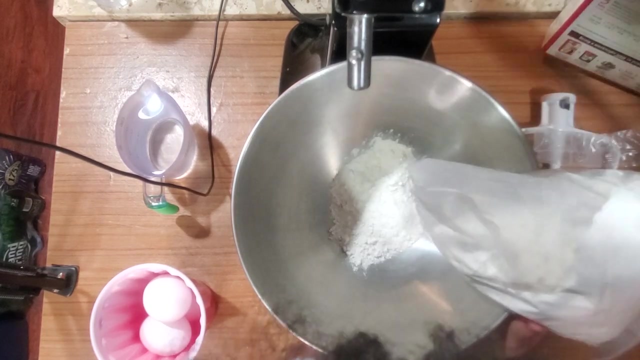 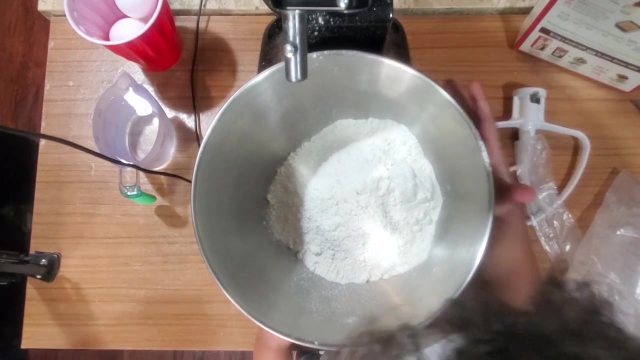 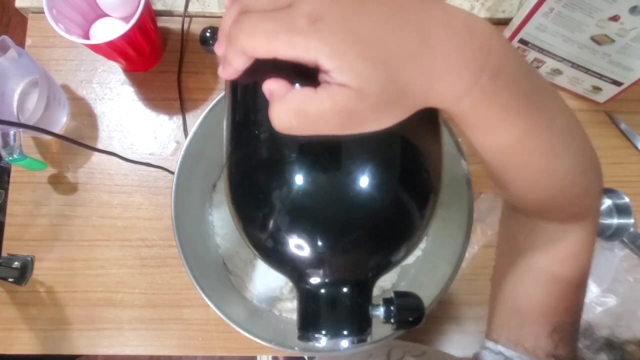 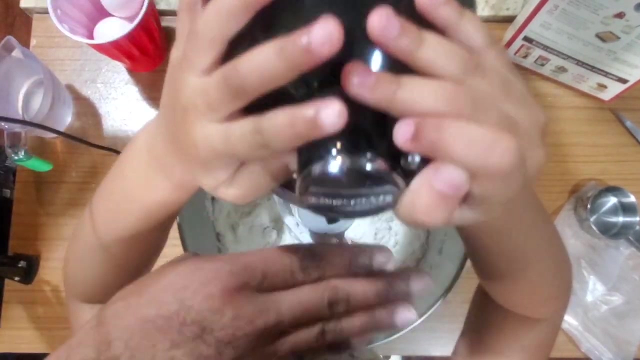 Okay, I'm going to pour it. I am going to let you, but Daddy's going to open it. okay. Okay, Daddy, Thank you. So here's the cake mix, Thank you. Now, what we're going to do is: 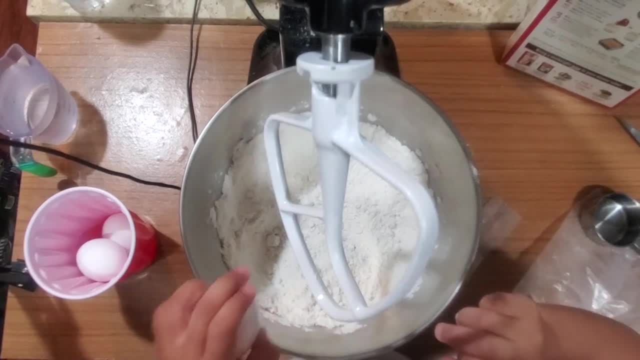 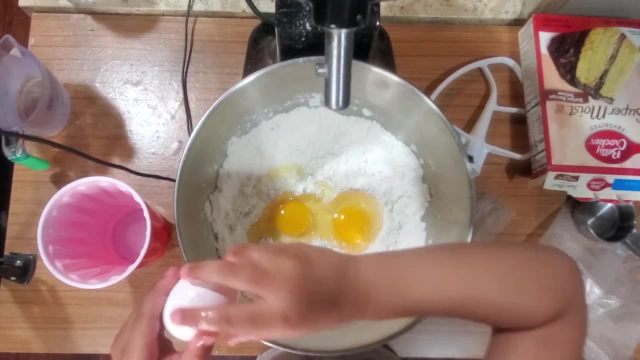 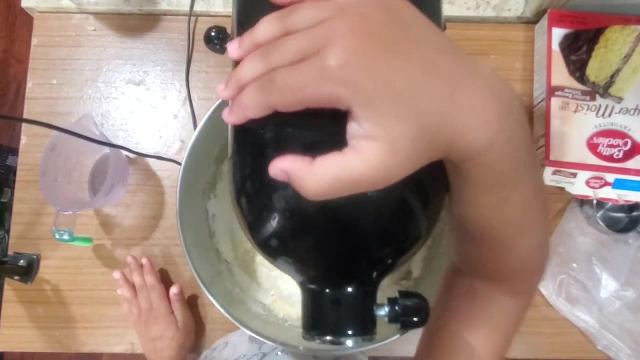 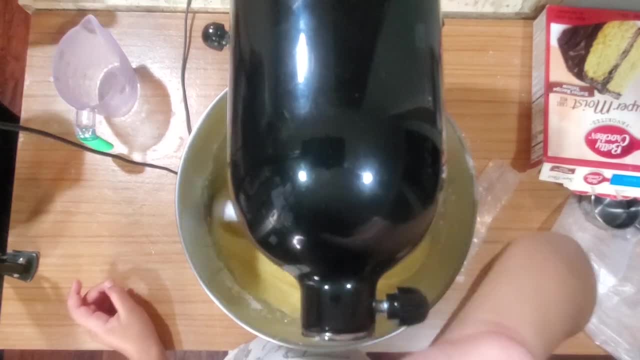 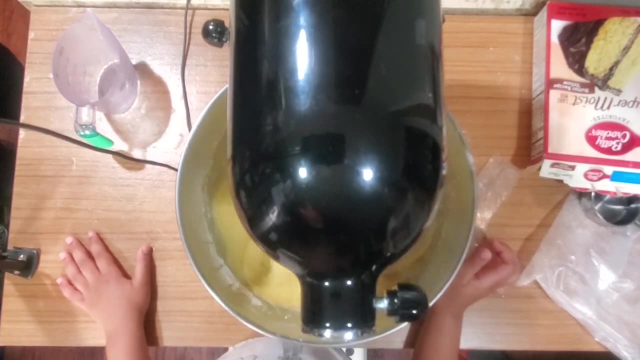 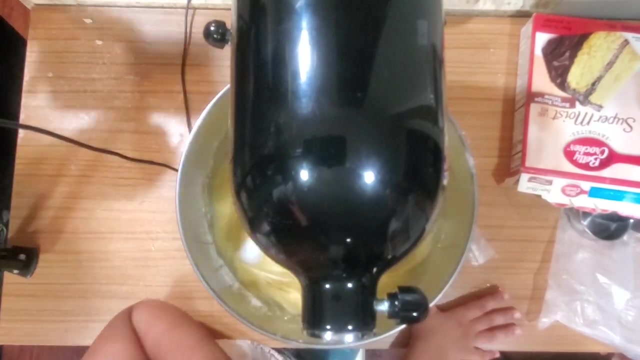 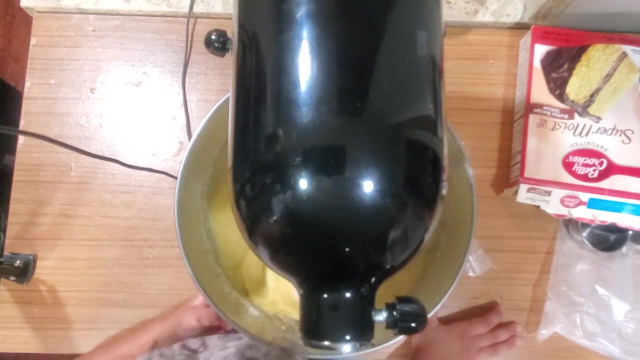 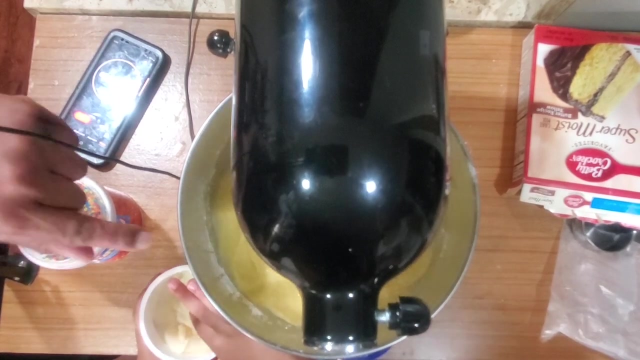 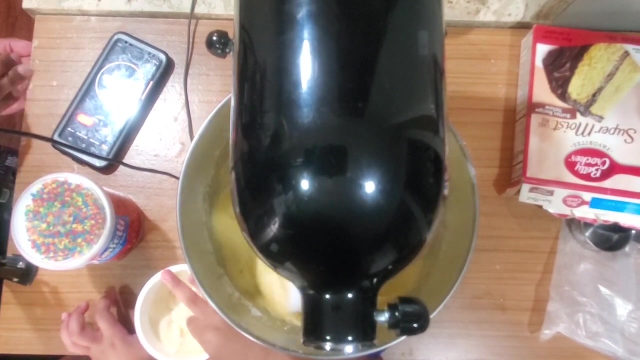 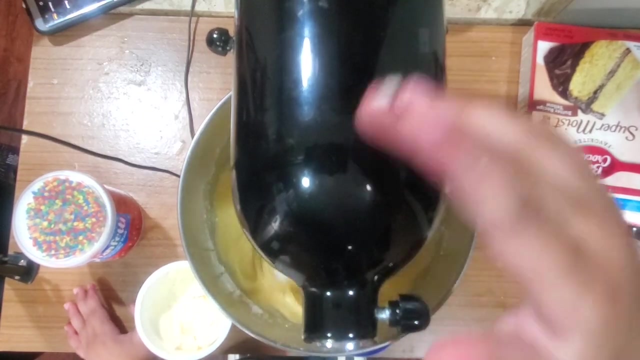 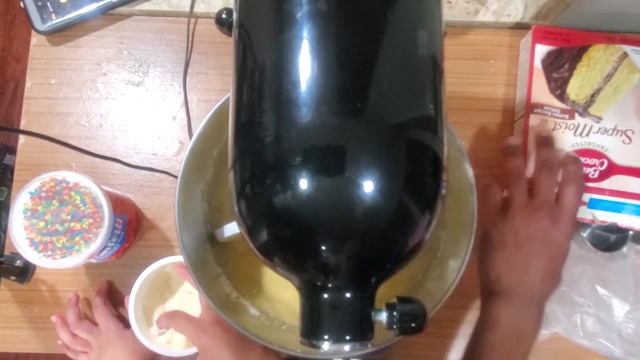 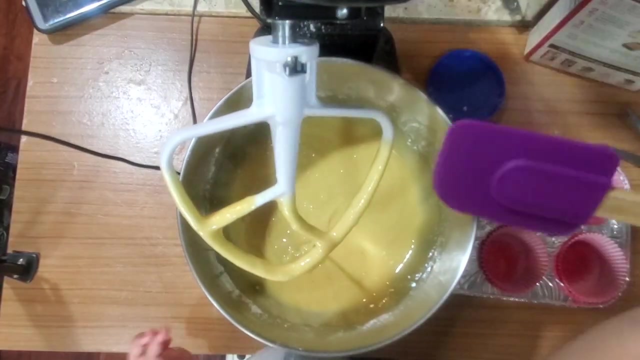 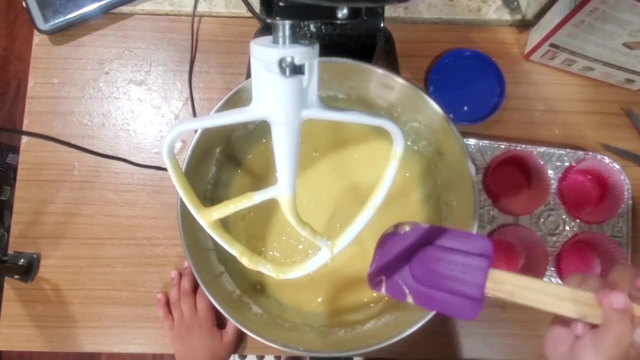 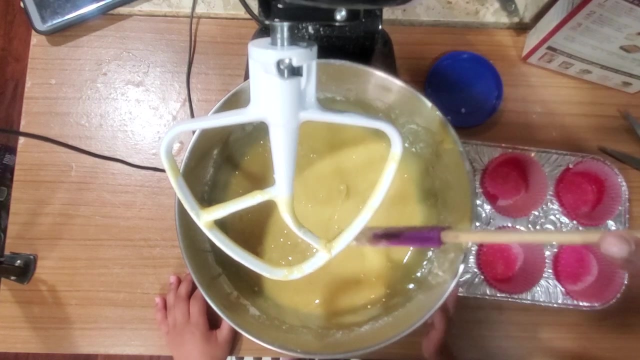 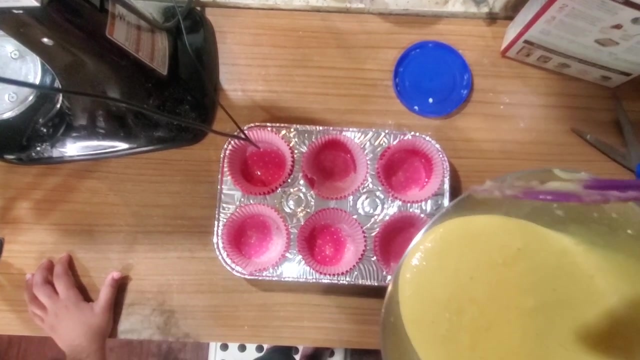 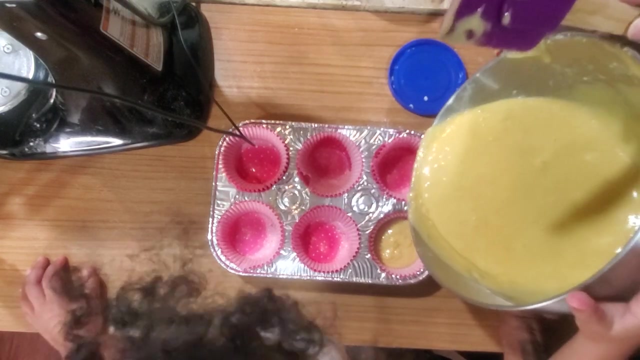 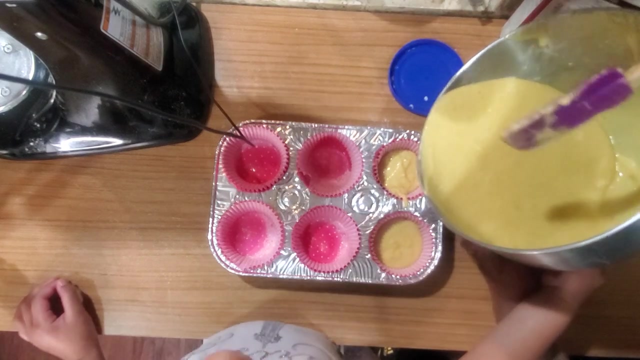 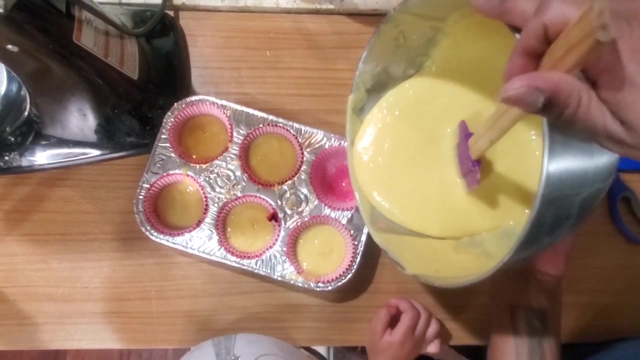 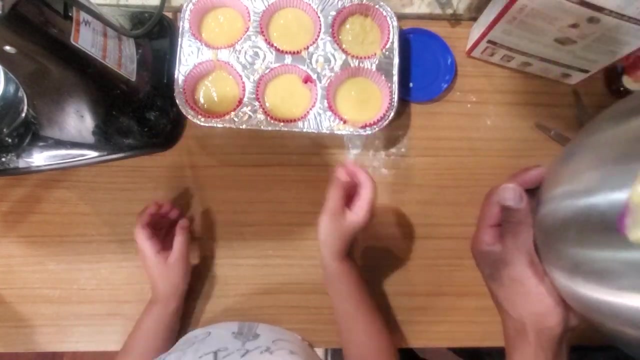 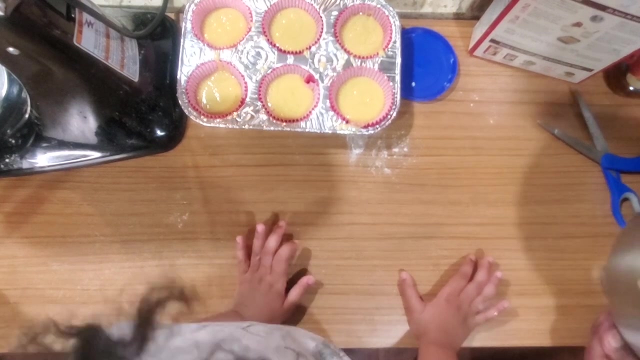 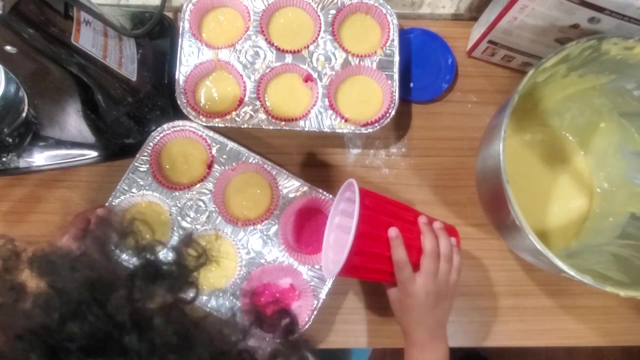 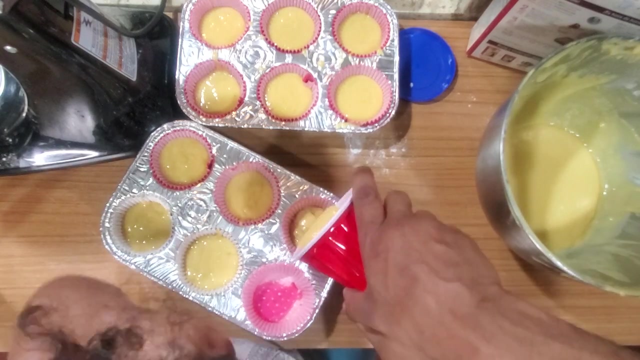 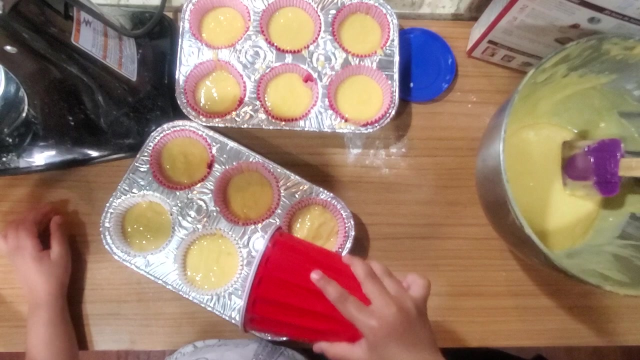 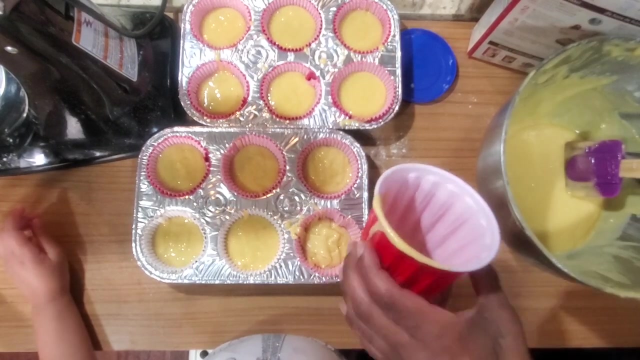 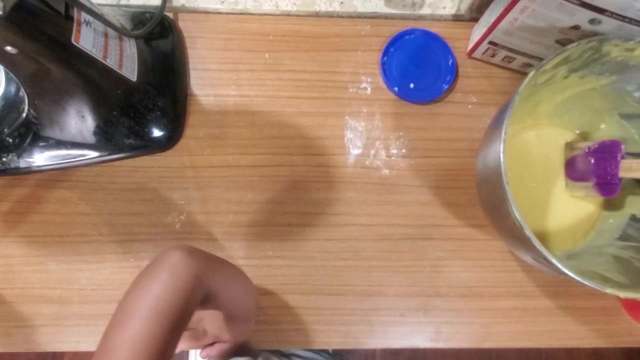 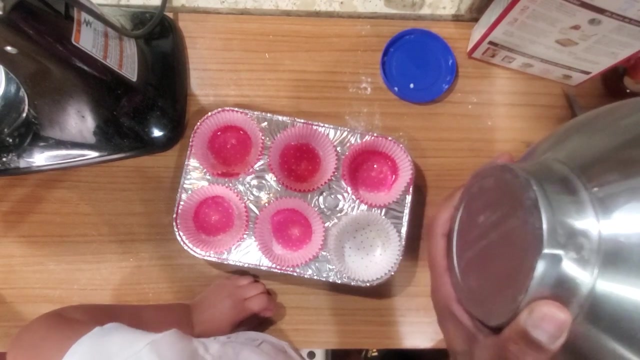 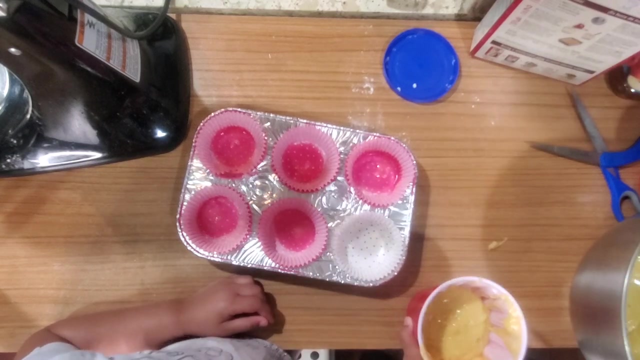 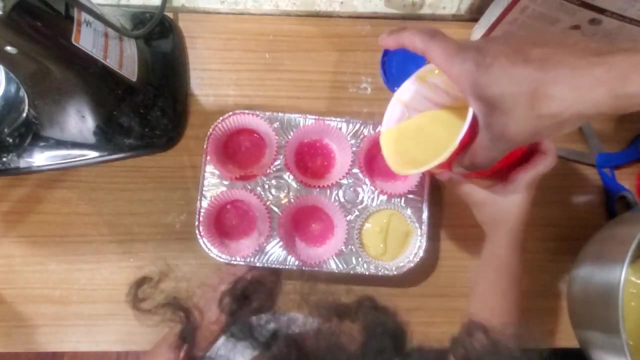 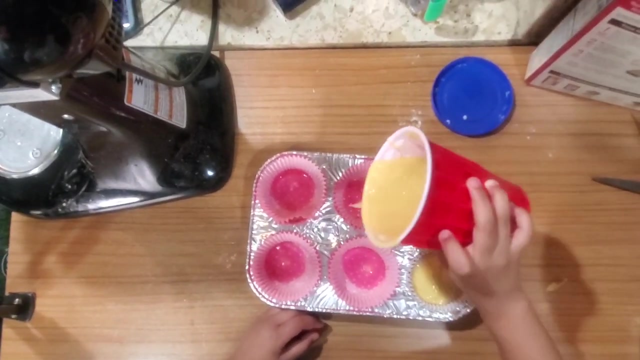 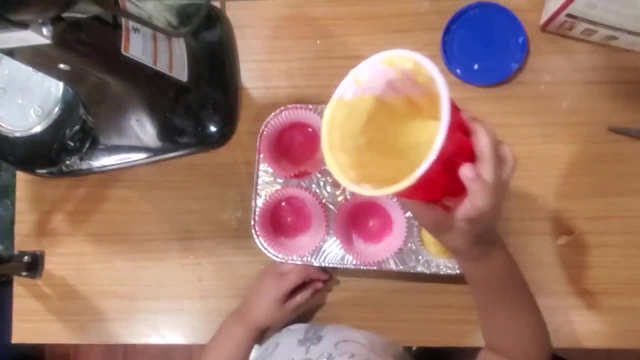 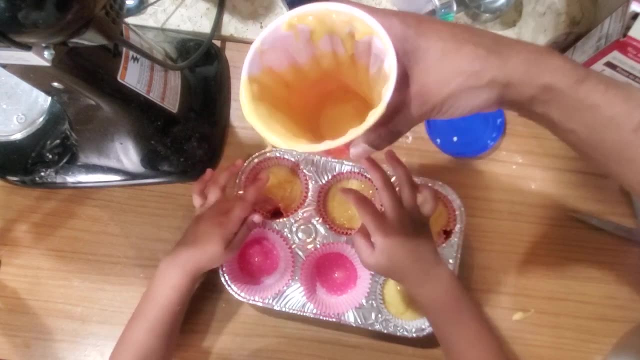 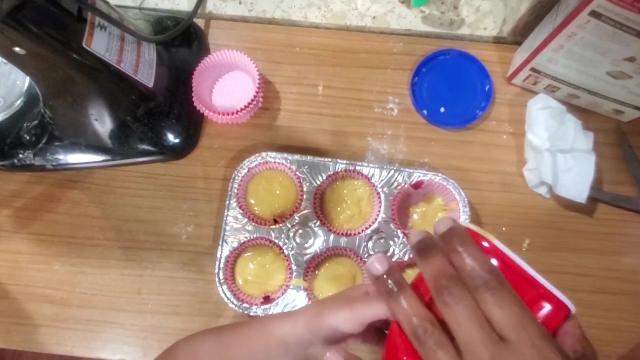 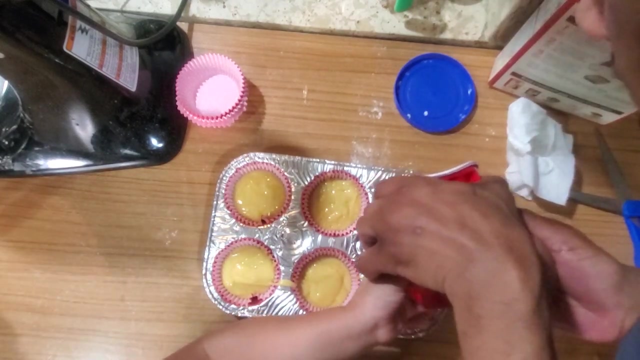 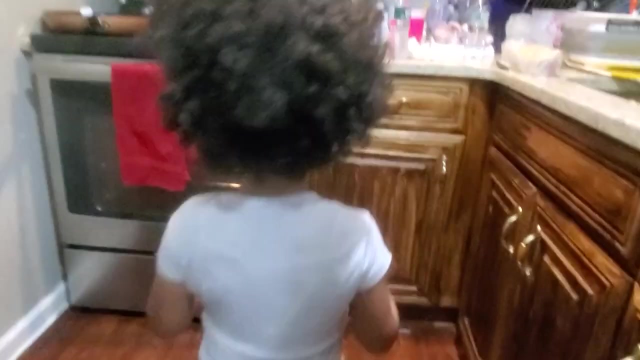 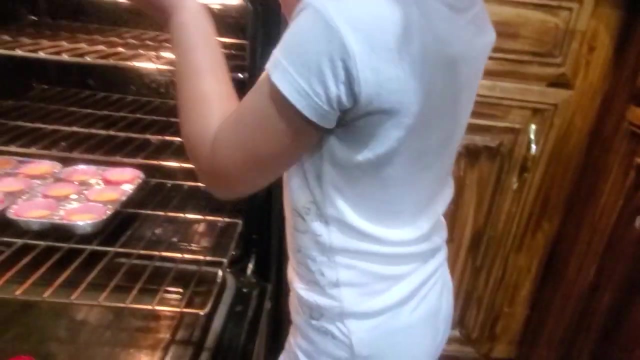 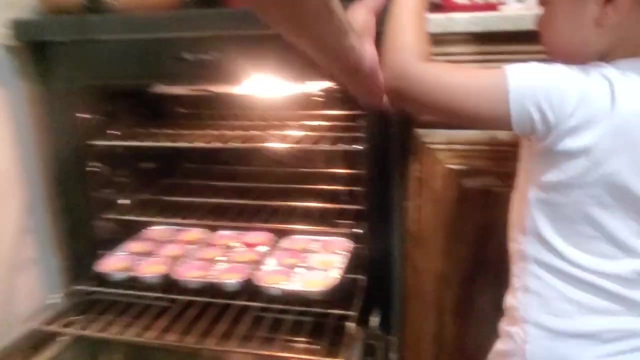 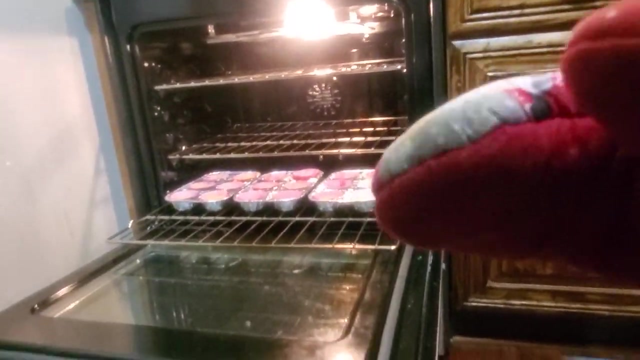 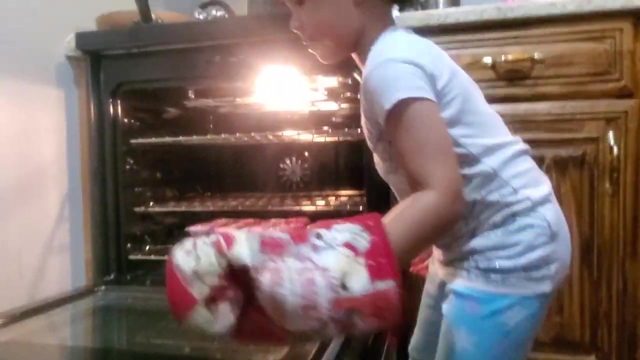 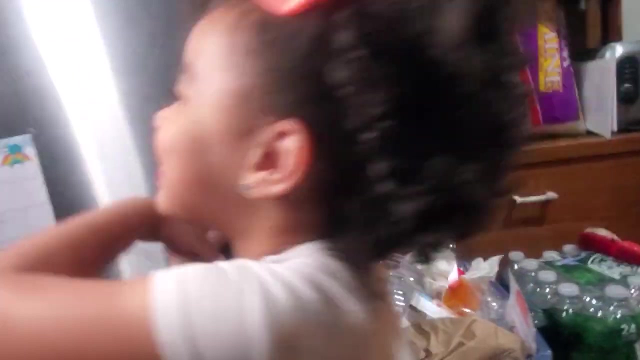 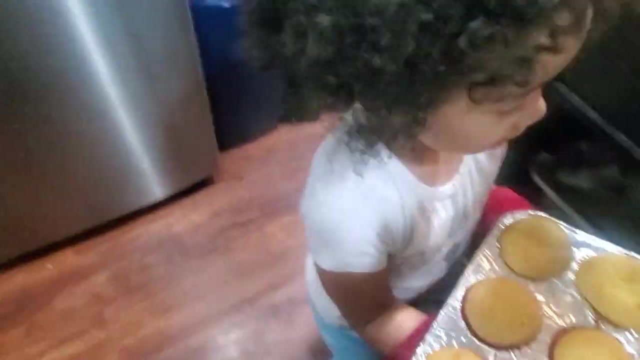 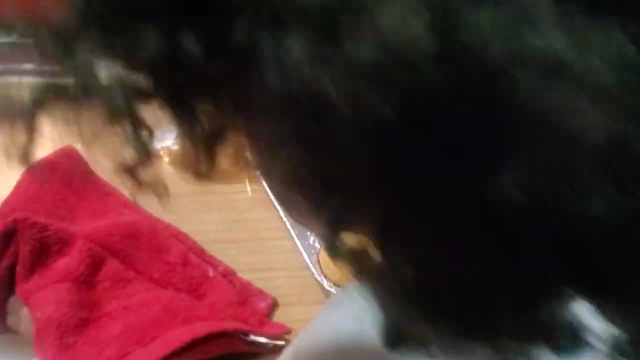 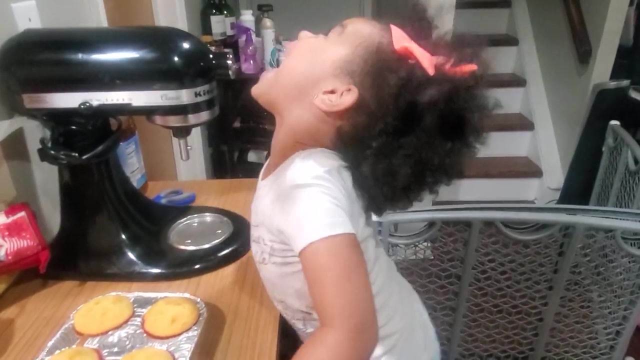 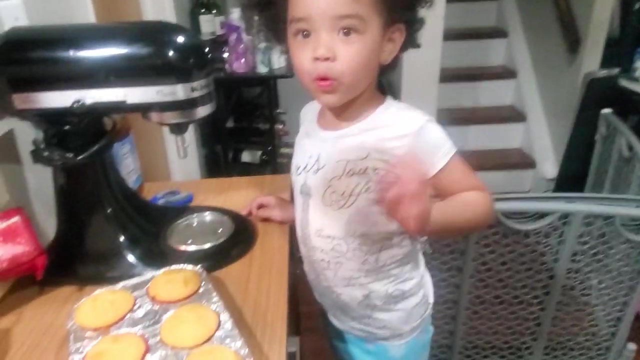 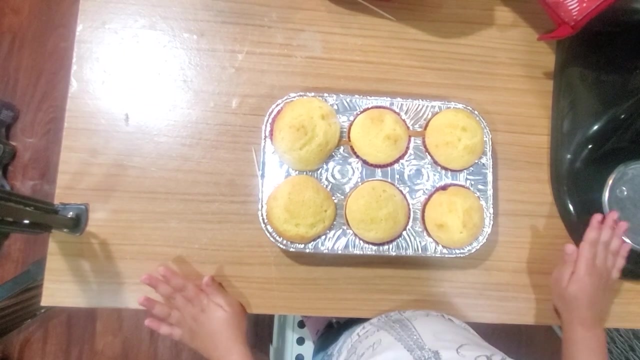 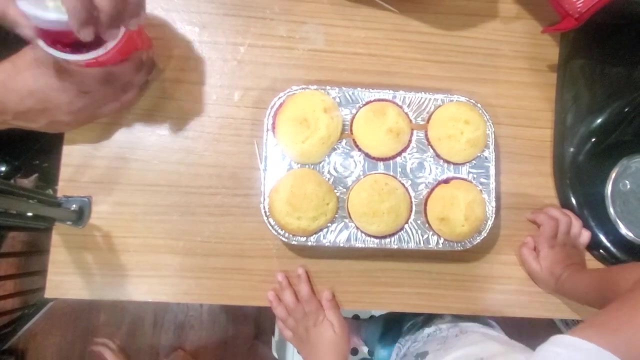